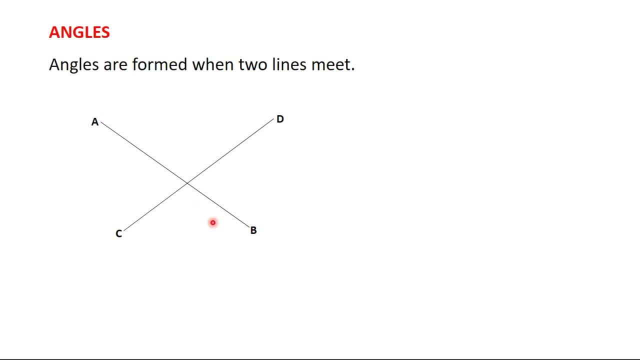 lines meet. When CD meets, AB angles will be formed. Now we are going to call their point of intersection the place that they meet. we are going to call their O. So the point of intersection that they meet, we are going to call their O. So we are calling this angle that we have here. 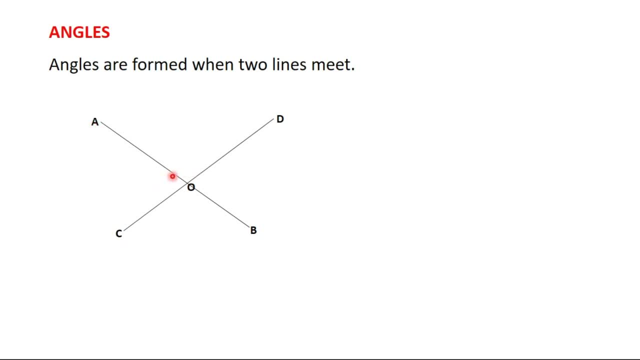 the angle formed between A and D. we are calling that angle angle M. Let's call it angle M, Let's call the one that we have here angle M, Let's call this angle X and let's call it here angle Y. Now I'm using these variables N, M, X and Y to represent the value, the actual. 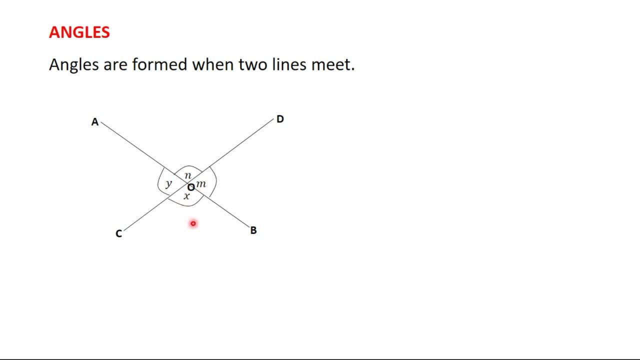 value of this angle. Now we are going to learn how to name an angle. An angle is named using the points that are forming the angle. So, for example, for angle M, for angle N- sorry, the points that are forming angle N are points A, O and D. So A, O and D are the points forming angle N. So the name of angle. 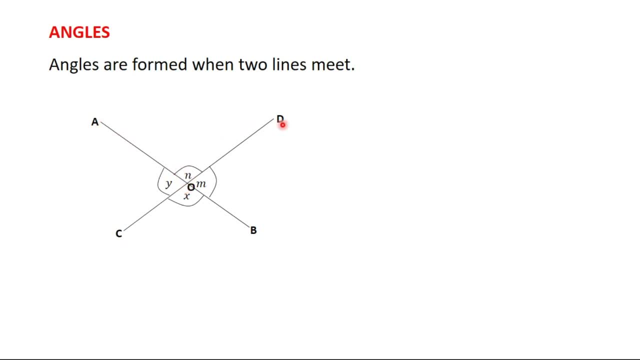 angle A, O, D or D O A. again, the name of this angle here, which is angle N, is angle A, O, D or D O A, because when naming the angle you use the points that form the angle, and always the point on which the angle falls must be in the middle. so here the angle is falling on point O. 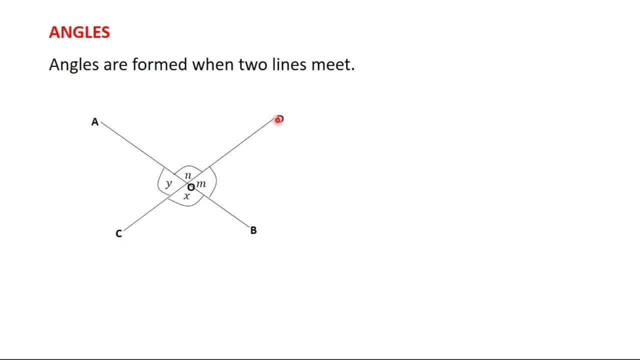 so the name is A O D or D O A and it's written as so. angle N: here we know that it's A O D or D O A. for simplicity's sake, I'm going to use A O D in this explanation. so angle A O D is written as this: 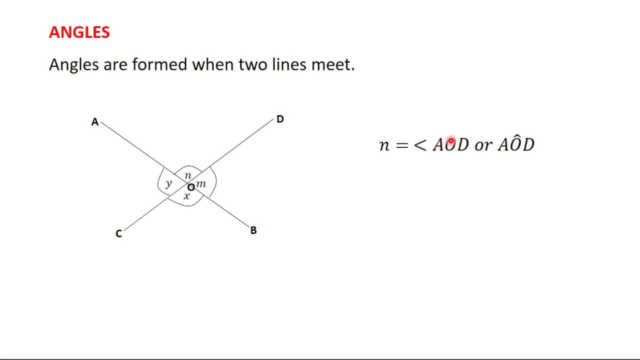 you write this less than symbol, then A O D or D O A, or you write A O D, then you make this sign on top of O, since the angle is on O. all that is clear. so this angle here, which is angle N, is called angle A O D or D O A, and it's written as: 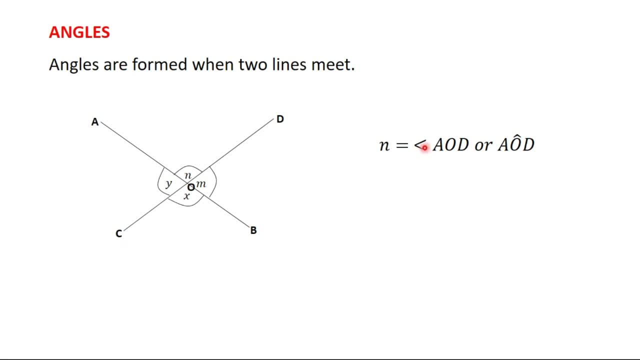 this sign here, this less than sign, which is read as angle. so angle A O D. or you write A O D or D O A, then you make this sign here on the point on which the angle is falling, which is point O. so A O D. then you make the sign on point O, all that is clear. 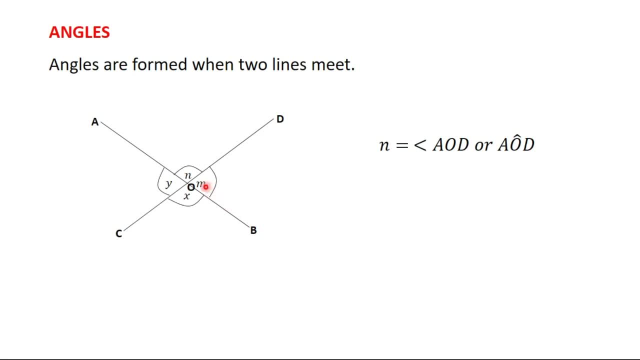 now let's move on to the next angle. you know that we call this angle here angle N, so to name this angle is going to be angle B, O D or D O B. it's still O because the point, the angle is falling on, point A O D. then you make this sign here, on the point on which the angle is falling, which is point O. so A O D, then you make the sign on point O. all that is clear. now let's move on to the next angle. you know that we call this angle here angle N, so to name this angle is going to be angle B O D or D O B. 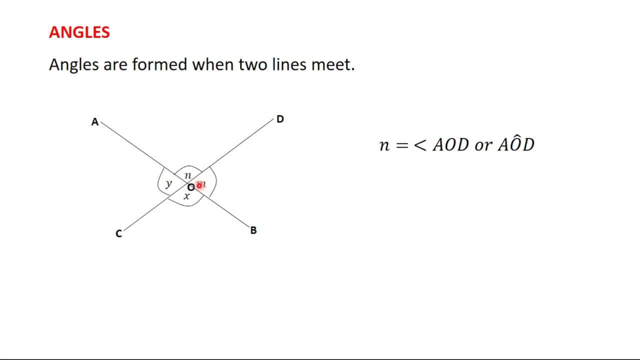 it's still O, because the point, the angle, is falling on the point O. so the name of this angle here, the angle from between D and B, is angle D O B or D B O D. it can be either one. the main thing that you have to make sure that happens is that 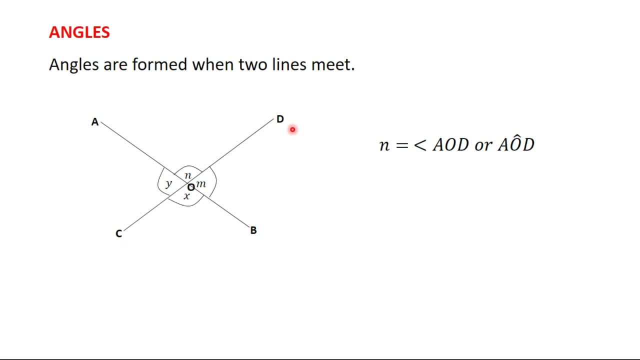 the point that the angle falls on must be in the middle. so this is angle B O D or angle D O B, And it's also written as angle BOD or BOD. then you bring the sign on top of it. Somebody can also choose to write angle DOB or DOB. then you bring the sign on top of the O. 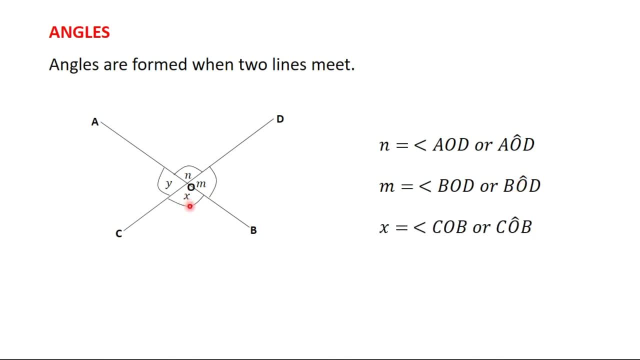 The same thing applies to what we have here as X. This is also angle COB or angle BOC. Now it's written as angle COB or COB, then with this accent on top of the O. Lastly, this angle is also angle AOC or angle COA. 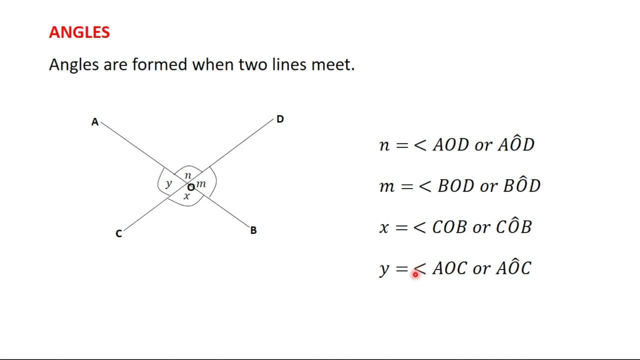 It's the same thing. All that you need to know is that this is how to write it, So you bring this sign here. angle: AOC or AOC, with this sign on top of the O. We are going to use this. 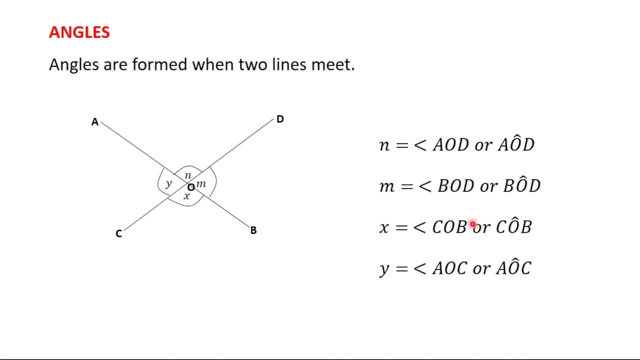 We are going to use this a lot in the subsequent videos that we should be considering, so we should be conversant with it So that when I mention an angle, let's say I mention angle AOC- you know that, the particular angle I'm talking about. 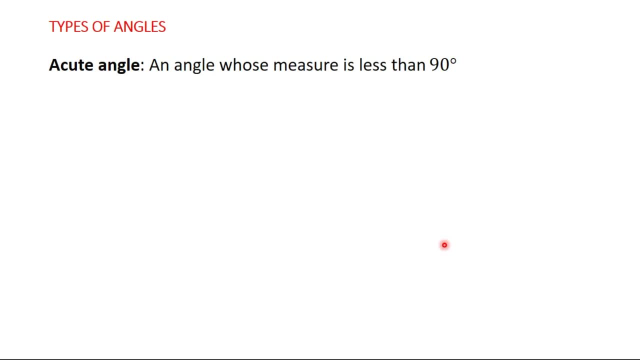 In this video we are going to also consider the types of angles. We learned so much about this in GHS, so we are going to go over it. We have one angle called acute angle, An angle whose measure is less than 90 degrees. 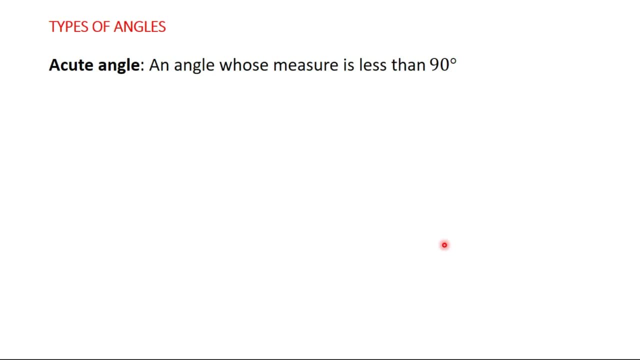 Angles are measured in degrees. so whenever you have an angle and the value of the angle is less than 90, we say that that angle is an acute angle. So, for example, 50 degrees is an acute angle, 20 degrees is an acute angle, 89 degrees is an acute angle. 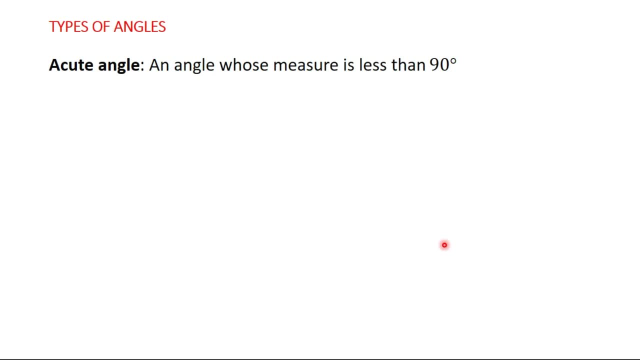 Any angle less than 90 degrees is called an acute angle. We have another one called the right angle, an angle whose measure is 90 degrees. So when you measure an angle and you get 90 degrees, that angle is called a right angle. 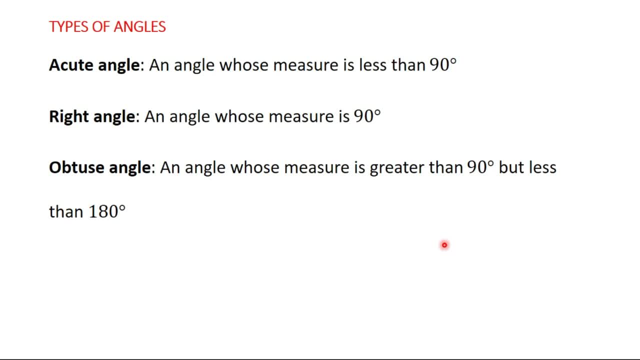 Another one is called an obtuse angle, An angle whose measure is greater than 90 degrees but less than 180 degrees. So if you have an angle whose value is greater than 90 degrees but less than 180 degrees- for example, 120 degrees- 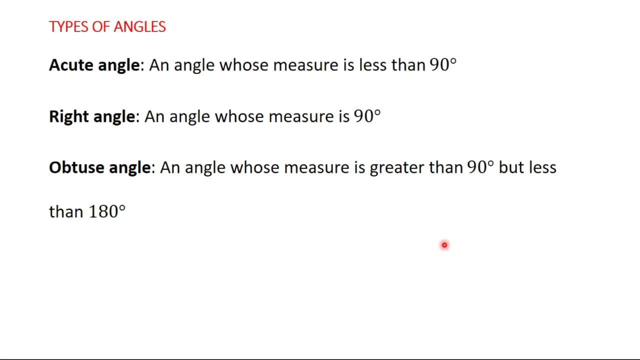 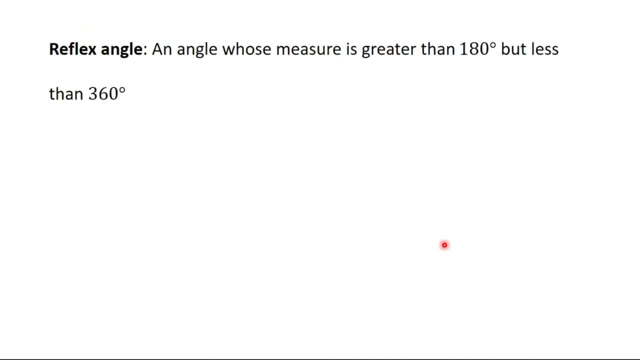 120 degrees is greater than 90 degrees but less than 180 degrees, We say that you have an Obtuse angle. Let's consider another type of angle called a reflex angle, An angle whose measure is greater than 180 degrees but less than 360 degrees. 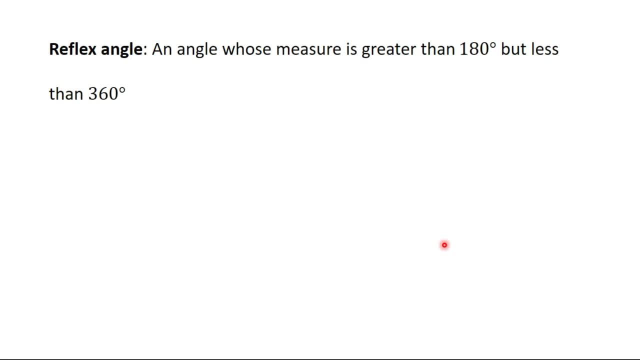 So an angle whose measure is greater than 180 degrees but less than 360 degrees is also a reflex angle. An example of that is 170 degrees. One Sorry Example of that is 170.. 270 degrees- Sorry. 270 degrees is greater than 180 degrees but less than 360 degrees. 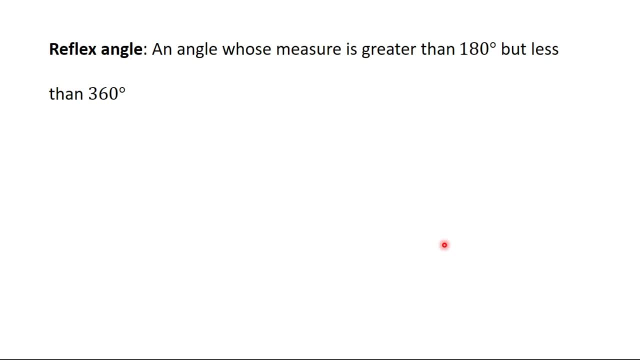 So we say that that is an example of a reflex angle. Then we have complementary angles, Two angles that add up to 90 degrees. So when you have two angles and you add them up and you are getting 90 degrees, we say that they are complementary angles. 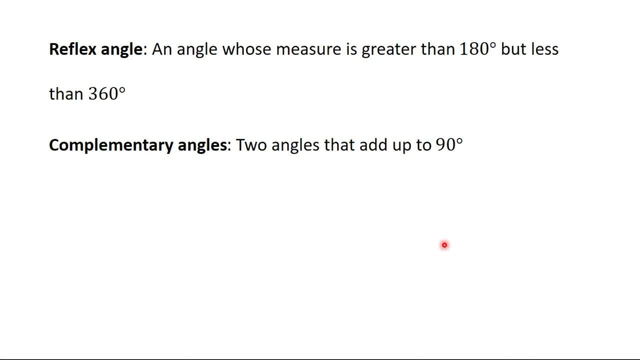 All that is clear. If you have two angles, you add those two angles and you get 90 degrees. Those two angles are said to be complementary angles. Then we have supplementary angles, Two angles that add up to 180 degrees. So if you have any two angles, you add them up and you are getting 180 degrees. 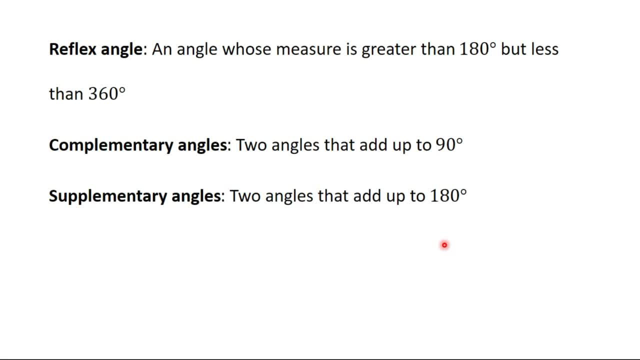 we say that they are supplementary angles. For example, if you add 60 degrees to 120 degrees, you are going to get 180 degrees. So we say that 60 degrees and 120 degrees are supplementary angles. We have learned about the types of angles. 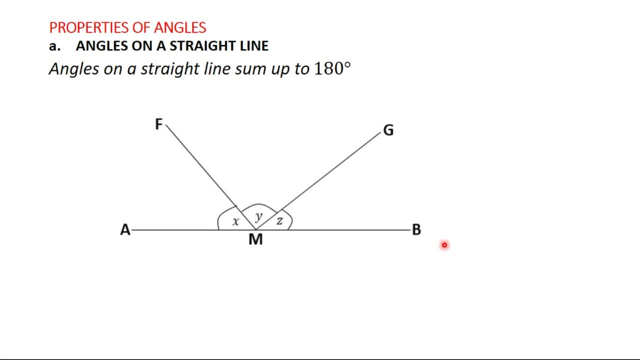 In this video also, we are going to learn about the properties of angles. Now pay attention to this very, very rule: Properties of angles. And the first property we are considering is angles on a straight line. Let's say we have this straight line, as we have here. 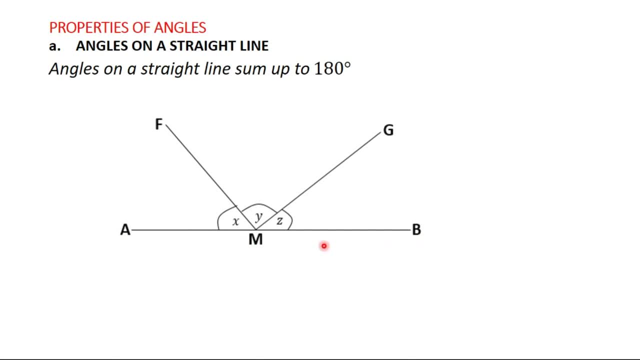 Line A M B, as we have here Now. this is the straight line. We have F Line F M joining line A B. Then we have line G M also joining line A B. Now you see, when that happens, you are going to create about three angles here. 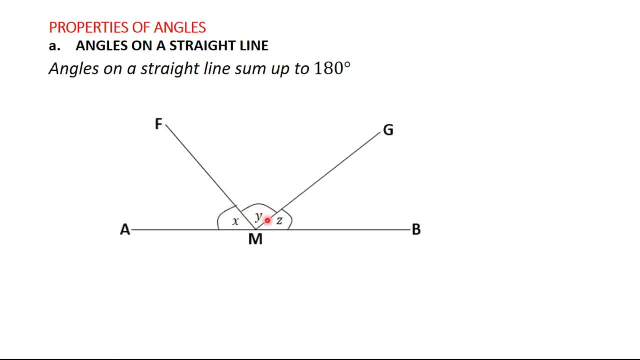 So we have this angle here which we are calling X, We have this angle here which we are calling Y, And we have this angle here which we are calling X. Now, this property states that angles on a straight line add up to 180 degrees. 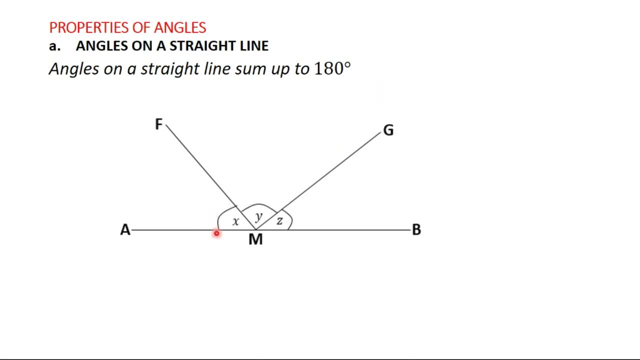 So, whenever you have angles on a straight line, if you add all of these angles, if you add all of these angles up, you are going to get 180 degrees. So what this means is that if we add X to Y, to Z, 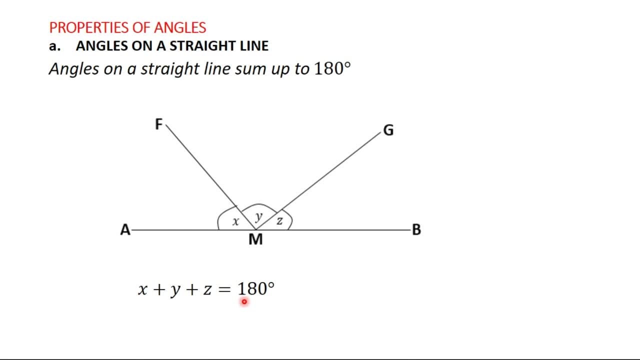 then we must get 180 degrees. This property of angles is very, very important. We are going to use it in the subsequent videos a lot, So make sure you get it. If you have a straight line and you add all the angles on a straight line. 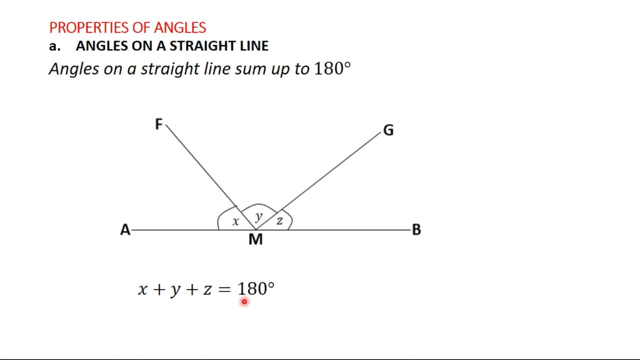 you must get 180.. Let's look at the next property. angles around a point sum up to 360 degrees. We learned in the previous slide that angles on a straight line add up to 180 degrees. This time it's not angles on a straight line, but angles around a point. 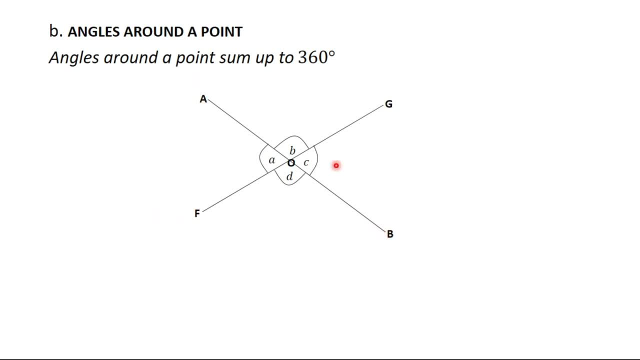 So we have line A, B and line F, G. they meet at a point called O. Now O becomes a particular point When you add all of these angles around a point. if you add all the angles around the point O, we are saying that you should get 360 degrees. 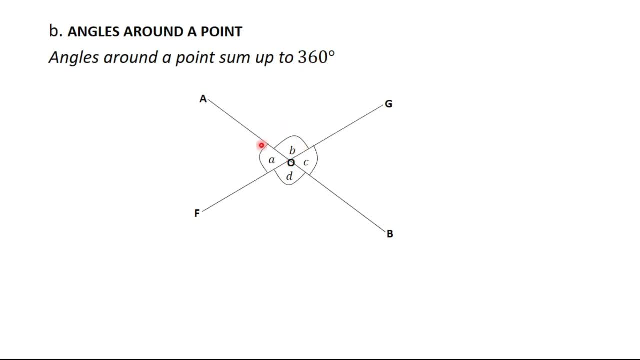 So, whenever you have a point, if you add all the angles around the point, if you add all of them, you must get 360 degrees. So what this means is that if you add A to B, you add that to C and you add that to D. 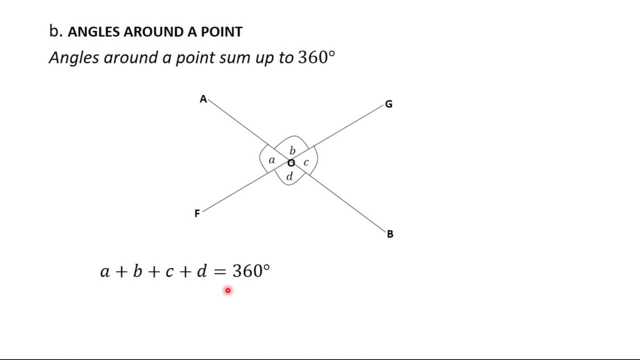 you must get 360 degrees. This is also very, very important. We are going to use it a lot as the video goes on. Let's look at the next property that we are considering: Vertically opposite angles. Let's say we have this line here, line P, S and line R K. 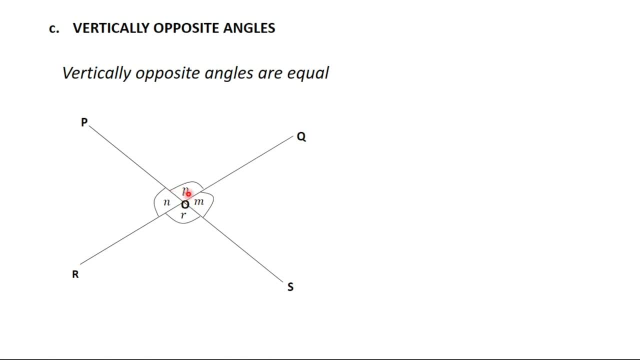 Now they meet at a point O. We have about four angles formed here. We can see from here that M is directly opposite to M, P is directly opposite to R. These are what we refer to as vertically opposite angles. So N is vertically opposite to M. 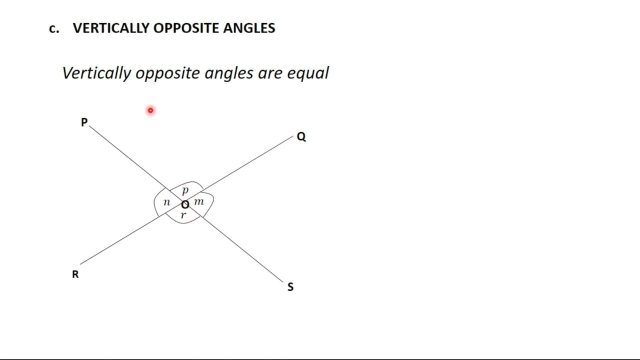 P is vertically opposite to R, And the property is telling us that vertically opposite angles are equal. It makes sense, right? So if P is directly opposite to R, then it makes sense that P is equal to R. N is also directly opposite to M. 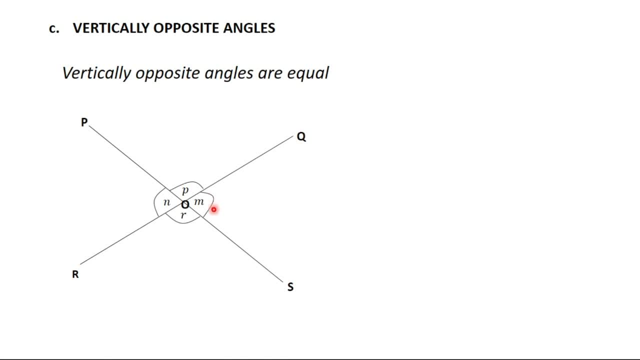 So we say that N is also equal to M. So we are saying that N is equal to M and P is equal to R. Remember, these are also angles around a point. So if you add all of them you should get 360 degrees. 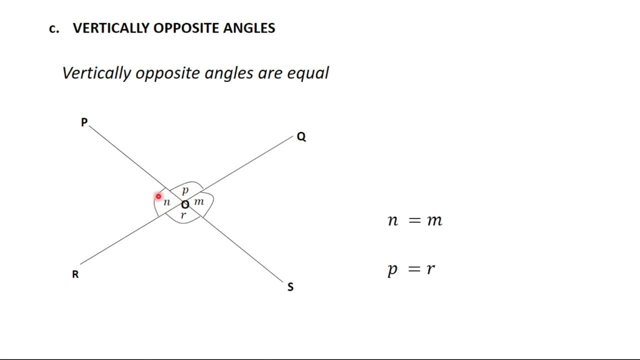 N and P are angles on a straight line, So if you add N and P, you should get 180 degrees. R and M are angles on a straight line, So when you add them you should get 180 degrees. But on this slide what you are considering are vertically opposite angles. 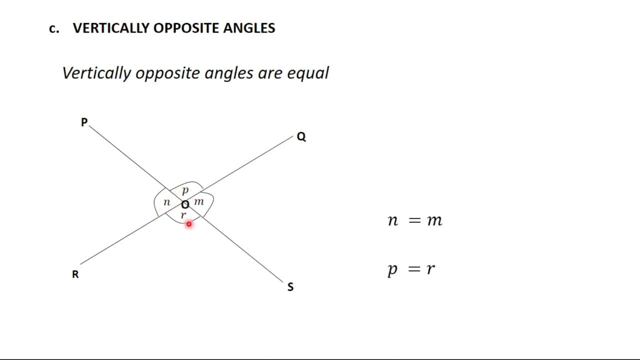 We know that P is vertically opposite to R, So P is equal to R, N is vertically opposite to M, So N is equal to M. This property is also very, very important And we are going to use it a lot. Let's look at the last property that we will be considering in this video. 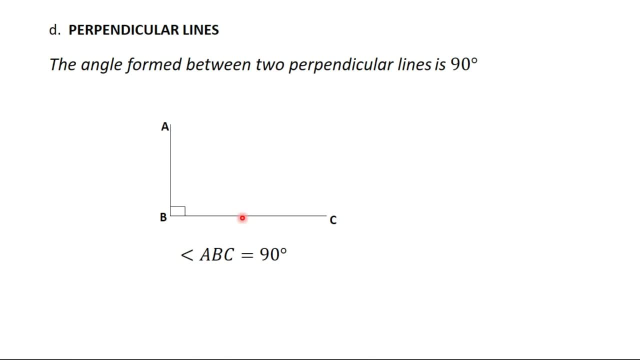 Angles formed between two perpendicular lines is 90 degrees. Now, when you have two perpendicular lines, in the video on menstruation and straight lines, we said that two lines are said to be perpendicular if they meet at 90 degrees. So in this case, line A B and line B C meet at 90 degrees. 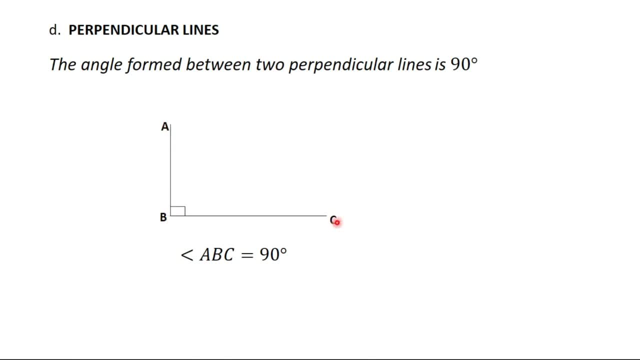 So we said that line A B and line B C are perpendicular to each other. We said that if you have two perpendicular lines and they are meeting, the angles formed between them is 90 degrees. So here the angle A, B, C. 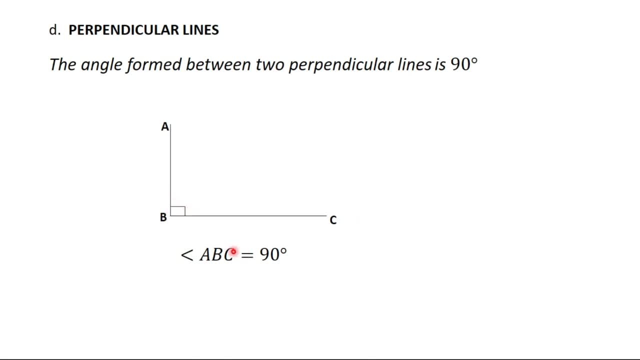 which is this angle we are talking about here- is 90 degrees. Now, whenever you see this sign, it means that the angle there is 90 degrees. So whenever you see this sign- now this is what I mean- If you have, let's say you have this line here. 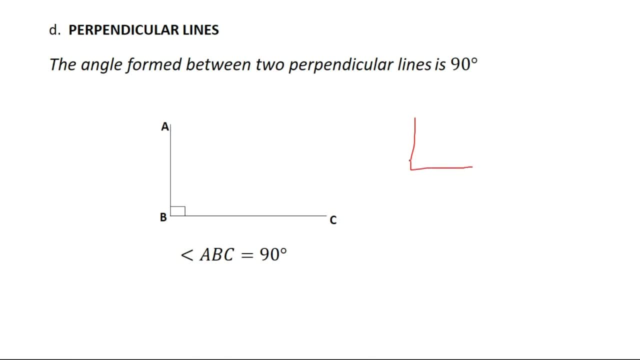 and you have another line and you see this sign in between them. it means that the angle formed around that particular area is 90 degrees. So here, the angle formed here is 90 degrees. So we've learnt about four properties. here We've learnt about the angles on a straight line. 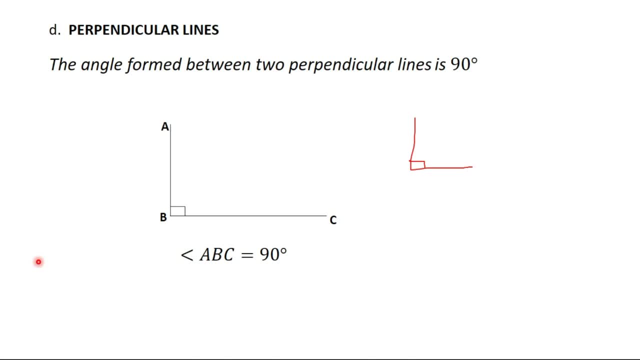 We know that they are equal to 180 degrees. We've learnt about the angles around a plant. We know that they are equal to 360 degrees. We also learnt that vertical opposite angles are equal, And we've learnt that the angles formed between two perpendicular lines is 90 degrees.